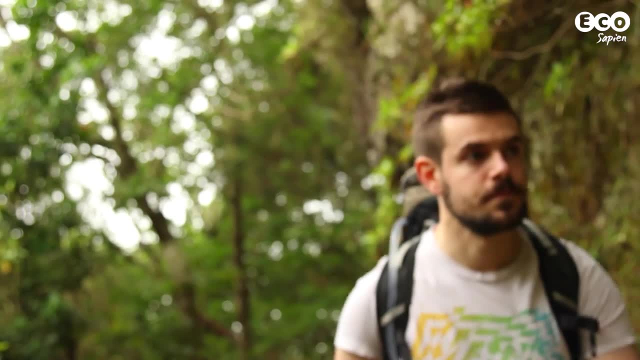 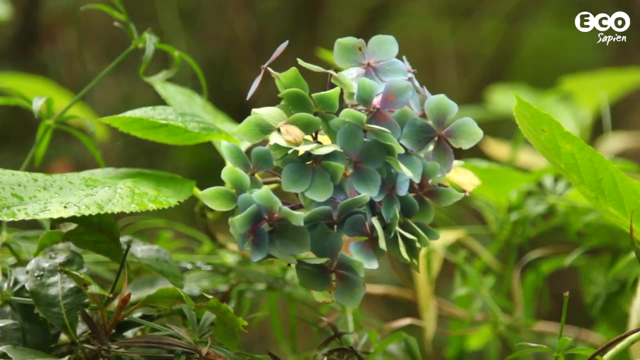 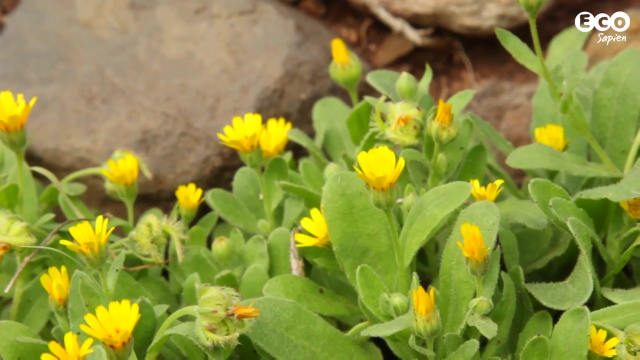 In actual fact, this forest is a relic from a time when similar vegetation covered the Mediterranean basin and was therefore designated a world heritage site in 1999.. Madeira is often referred to as the floating garden, and no wonder, For an island only 801. 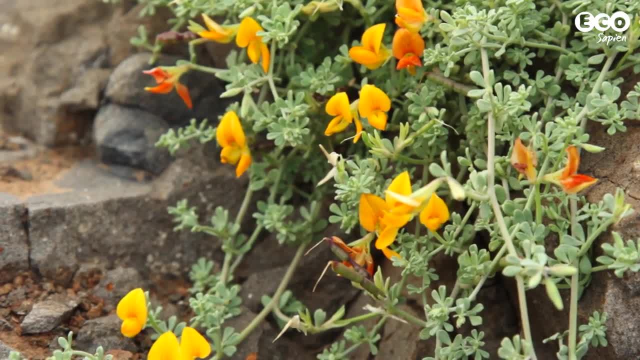 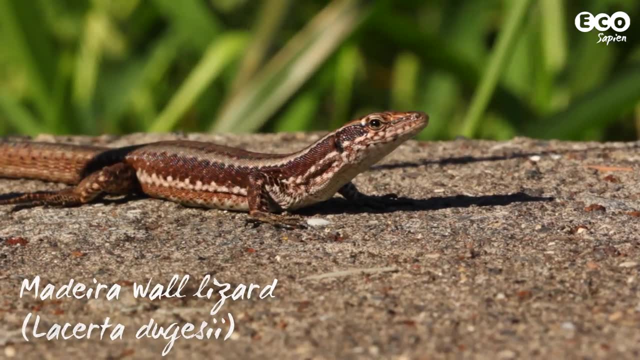 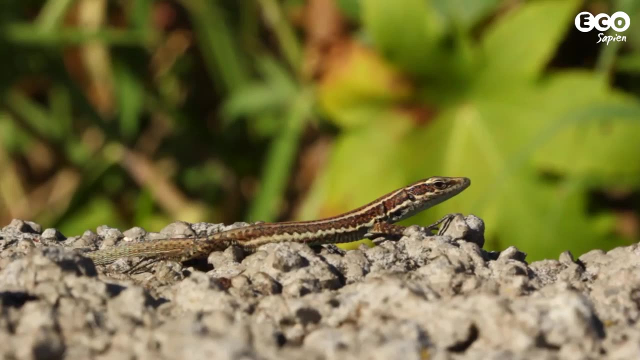 kilometers in area. it's home to over 760 species of plant. 140 of these are endemic. The island is also home to an endemic lizard, which is actually very common. It can be found on most walls and rock faces around the island. So why does Madeira have so many endemic species? Well, 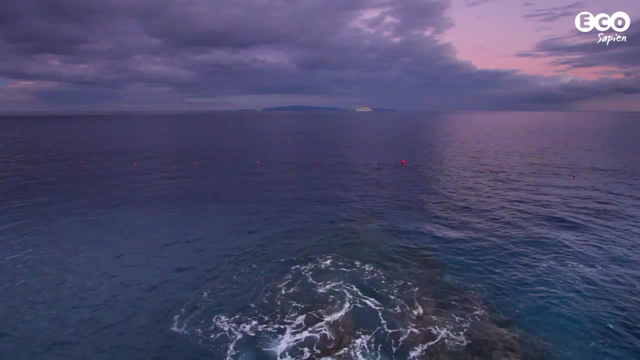 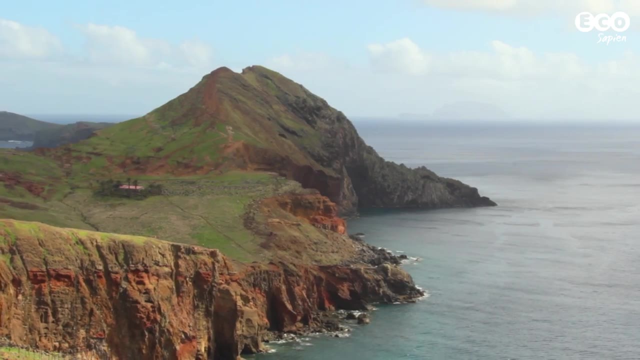 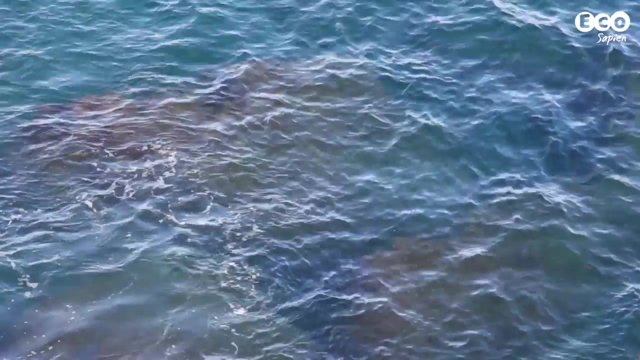 let's look at the ecological processes involved. Separated from continents by miles of water makes islands pretty isolated, Like Madeira. oceanic islands are formed by volcanic activity or even coral reef growth. This new patch of land is open to colonization and exploitation by organisms. 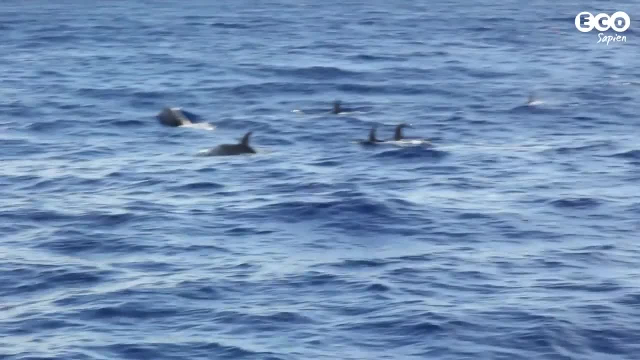 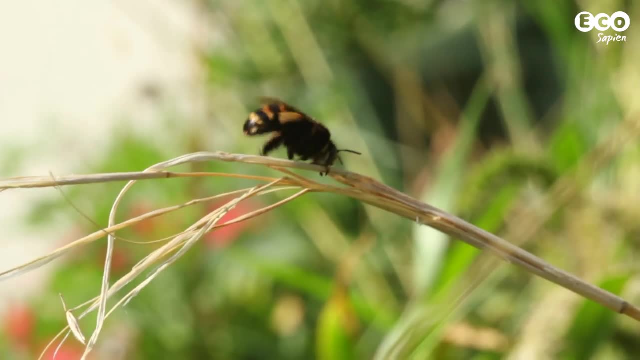 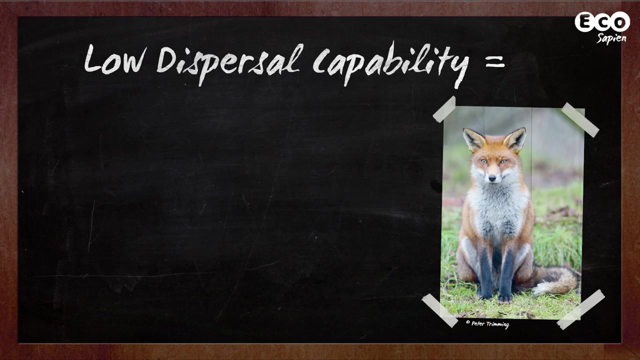 The trouble is, the only way to reach the island is by sea flight or even being blown over by the wind. This means organisms with a high dispersal capability, ie plants and birds, are much more common on islands, So animals like mammals that have a poor dispersal capability rarely make it. 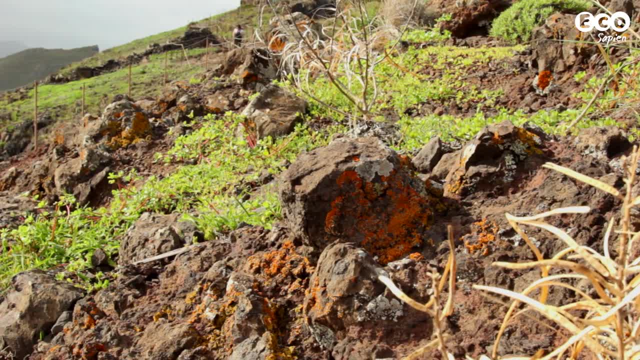 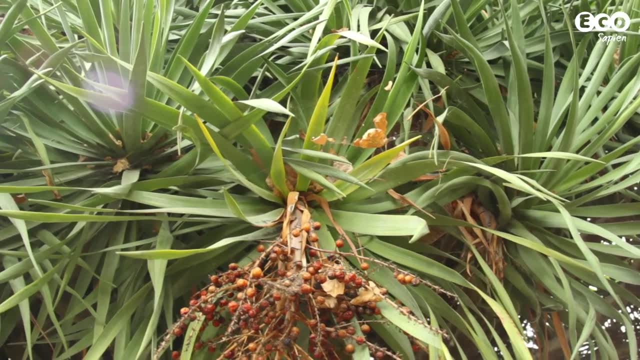 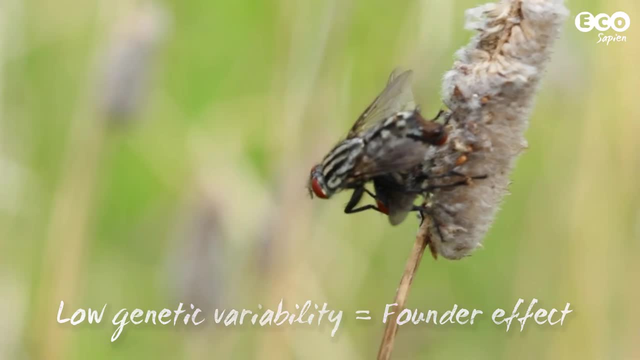 to isolated islands. Over time, ecological succession takes place. Some species that arrive survive and form populations. Because of the isolation, islands tend to be much less biodiverse than mainland ecosystems and exhibit low genetic variability. But there is an upshot of the isolation Void of traditional 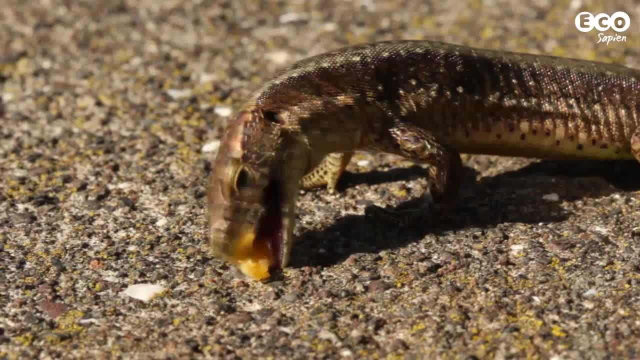 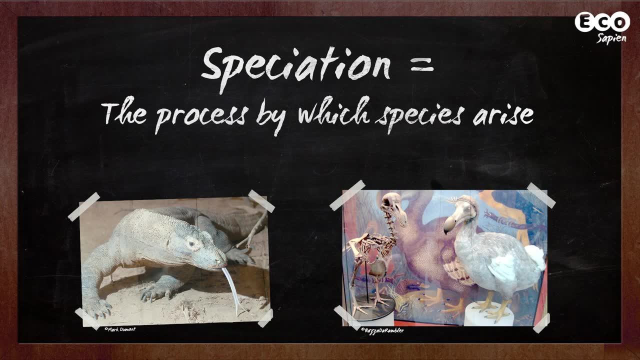 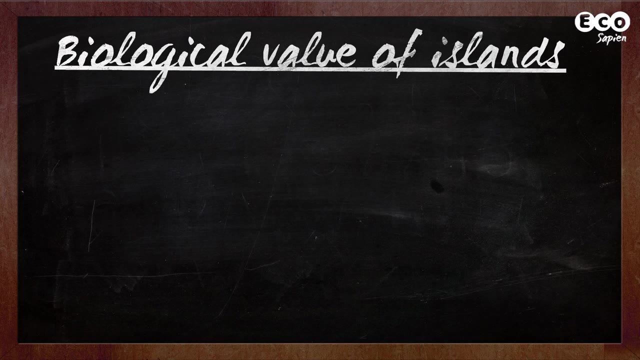 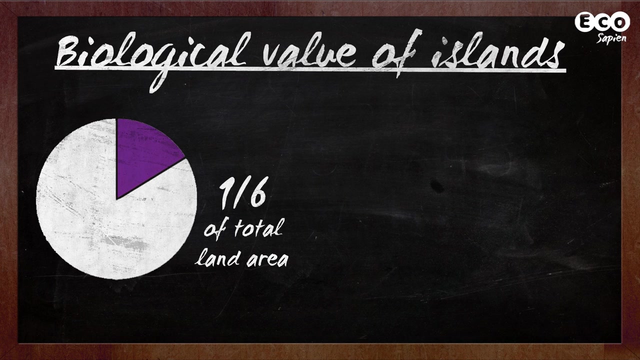 predators and competitors that species might have previously evolved with, they take advantage of new niches. As a result, the island is more and more isolated. Species are often unique to an island or a group of islands. As biodiversity goes, islands are extremely important, making up a sixth of the earth's total land area And, as a result of their